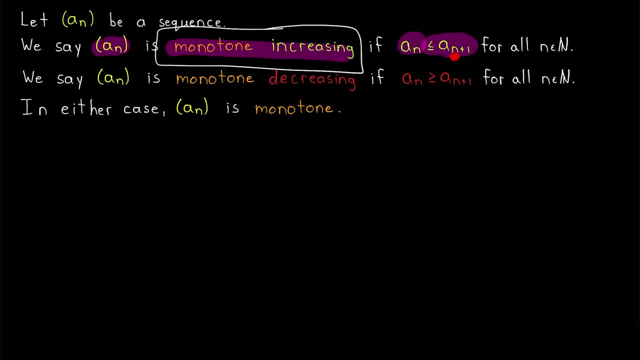 up, Each term is less than or equal to the next one. Similarly, we say that a? n is monotone decreasing if each term a n is greater than or equal to the next term, a n plus one. So in a decreasing sequence, each term can either stay the same or decrease, because each term is 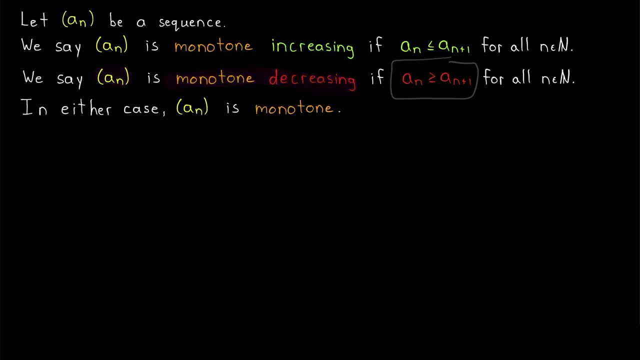 greater than or equal to the next one. If a sequence is monotone, increasing, we'll often just say that it is increasing. Similarly, we would just say that a sequence is decreasing. In either case, the sequence is considered monotone. So if we just say that a sequence 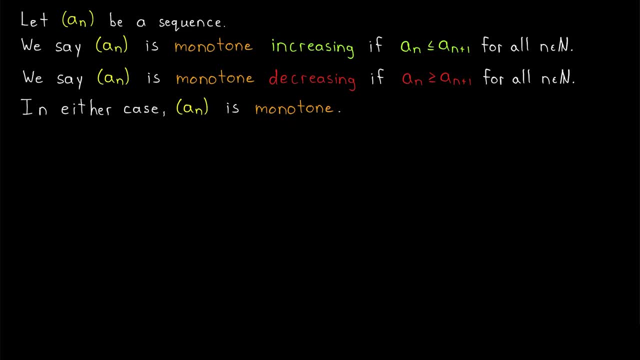 is monotone, then it is increasing or decreasing. But one weird thing we should quickly point out about this definition: Is this a sequence that we might represent like this, just a sequence of ones? Is this a monotone sequence? Indeed, it is In this sequence. we have that a n equals one. So we have that a n. 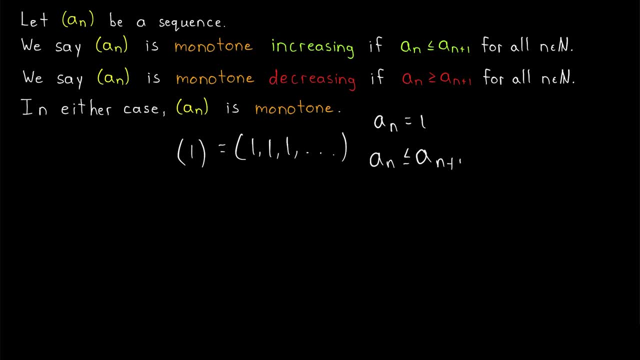 is certainly less than or equal to a n plus one for every n, because every term happens to be equal to the next term. But similarly we have that each term a n is less than or equal to a n plus one is greater than or equal to the next term, since, again, they're all equal. Thus a sequence. 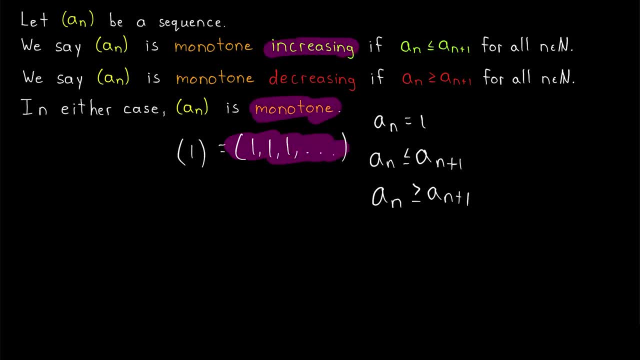 like this is monotone. it is increasing and it is decreasing. Of course it's a little weird to have a sequence that we consider increasing and decreasing, But there's no compelling reason to exclude constant sequences from these definitions, So we don't. Here's another example for you. 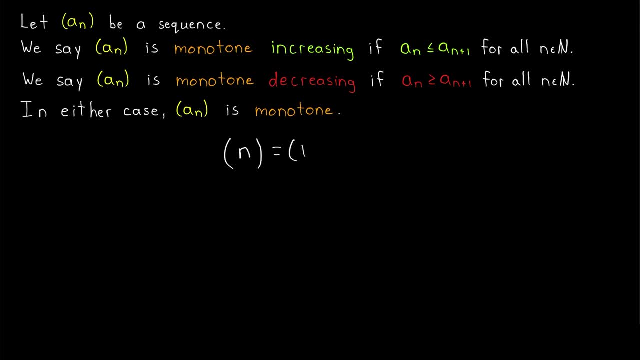 consider this sequence where the nth term is equal to n. is this sequence monotone? Indeed, this sequence is monotone. it happens to be increasing because each term, a n is one less than the next term. So, certainly, every a n is less than or equal to a n plus one. each term is less than or equal to the next one, And so 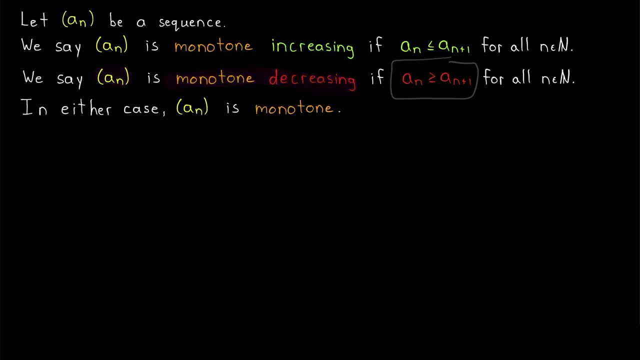 greater than or equal to the next one. If a sequence is monotone, increasing, we'll often just say that it is increasing. Similarly, we would just say that a sequence is decreasing. In either case, the sequence is considered monotone. So if we just say that a sequence 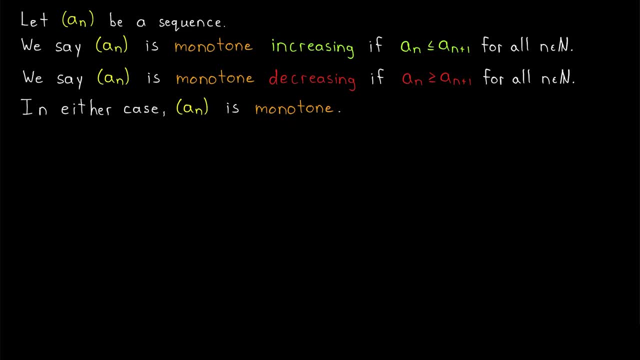 is monotone, then it is increasing or decreasing. But one weird thing we should quickly point out about this definition: Is this a sequence that we might represent like this, just a sequence of ones? Is this a monotone sequence? Indeed, it is In this sequence. we have that a n equals one. So we have that a n. 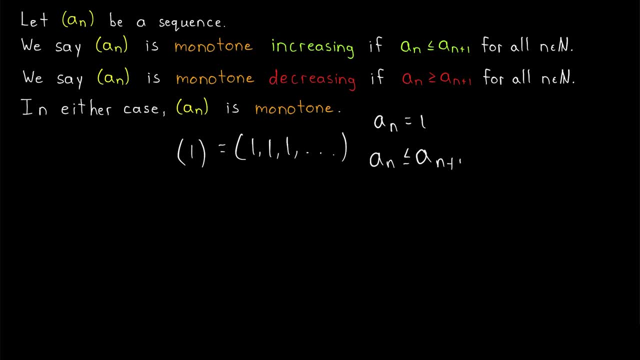 is certainly less than or equal to a n plus one for every n, because every term happens to be equal to the next term. But similarly we have that each term a n is less than or equal to a n plus one is greater than or equal to the next term, since, again, they're all equal. Thus a sequence. 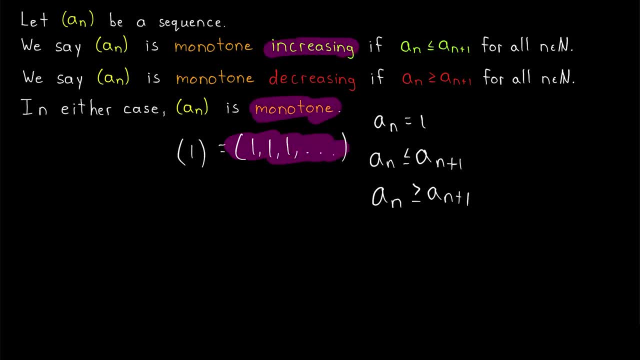 like this is monotone. it is increasing and it is decreasing. Of course it's a little weird to have a sequence that we consider increasing and decreasing, But there's no compelling reason to exclude constant sequences from these definitions, So we don't. Here's another example for you. 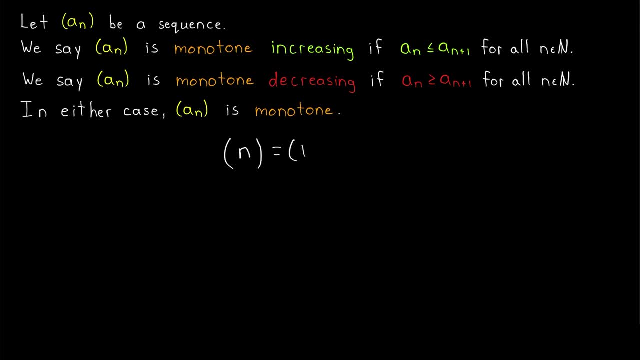 consider this sequence where the nth term is equal to n. is this sequence monotone? Indeed, this sequence is monotone. it happens to be increasing because each term, a n is one less than the next term. So, certainly, every a n is less than or equal to a n plus one. each term is less than or equal to the next one, And so 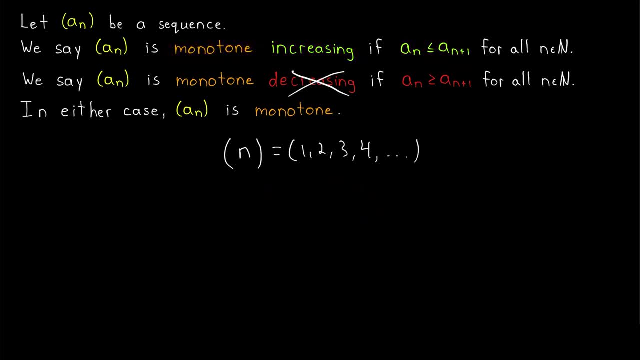 it is increasing. It's certainly not decreasing because, for example, the first term, a n, is less than the next term, a n is two. And remember, in a decreasing sequence, every term has to be greater than or equal to the next one. Now, how about this sequence? 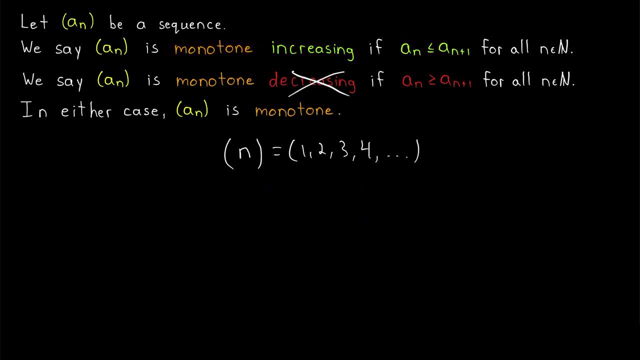 it is increasing. It's certainly not decreasing because, for example, the first term, a one, is less than the next term, a two. And remember, in a decreasing sequence, every term has to be greater than or equal to the next one. Now, how about this sequence? 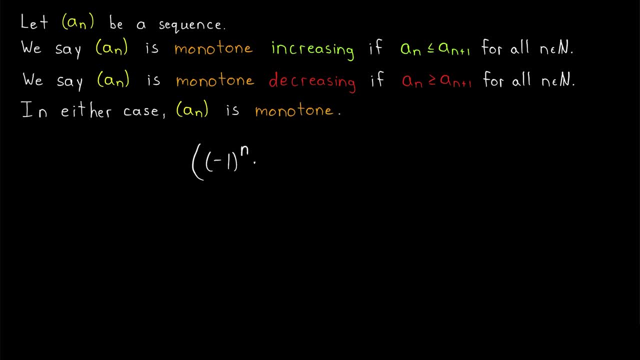 where the nth term is equal to negative one, to the power of n times n. the terms of this sequence are negative one, then positive two, then negative three, then positive four, 4 and so on. This sequence certainly isn't increasing since, for example, the second term 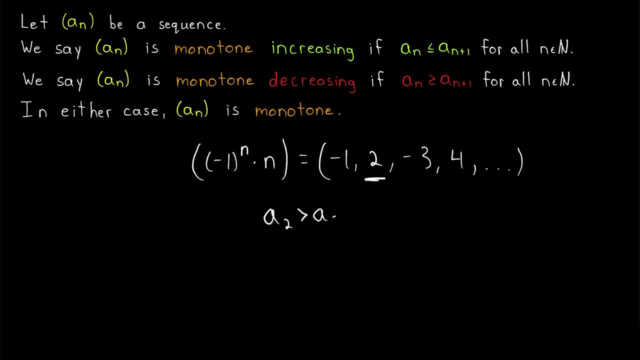 a2 is greater than the third term, a3, and to be increasing every term has to be less than or equal to the next one. Similarly, this sequence cannot be decreasing because, for example, the first term, a1, is less than the second term, a2, and for a sequence to be decreasing every term. 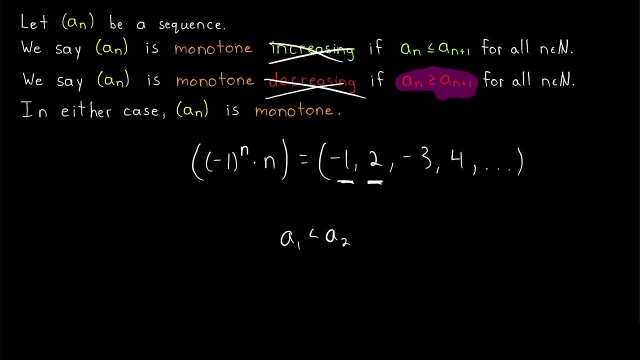 has to be greater than or equal to the next one. So this sequence is not monotone. How about the sequence where the nth term is equal to one over n? So the terms of this sequence are one over one, then one over two, then one over three, and so on. In this case, every term. 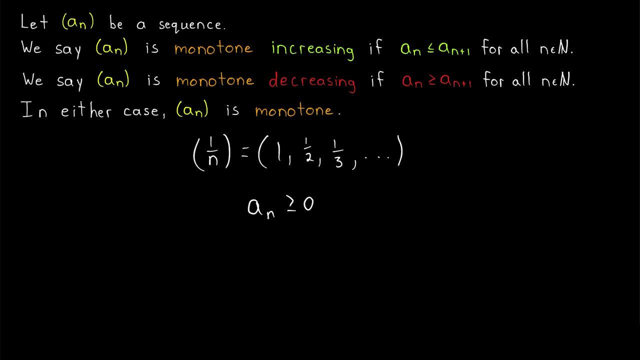 is greater than or equal to a2.. So this sequence is not monotone. How about the sequence where the a n is indeed greater than or equal to the next term, a n plus one, And so this sequence is decreasing? we could prove that by noting that n plus one is greater than n, and then invert both. 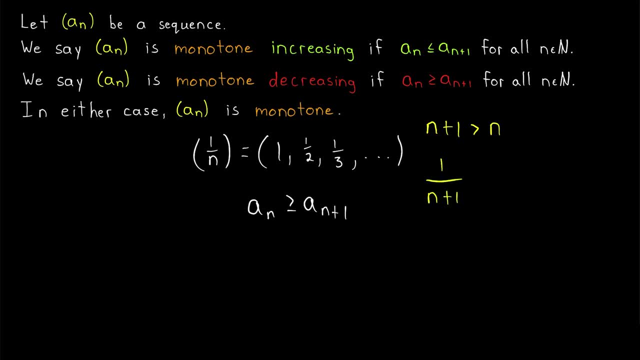 sides of the inequality, giving us that one over n plus one is less than one over n. And then this is the definition of a n plus one. this is the definition of a n, and we'd have that each term a n is greater than a n plus one. So certainly a n is greater than or equal to a n plus one. 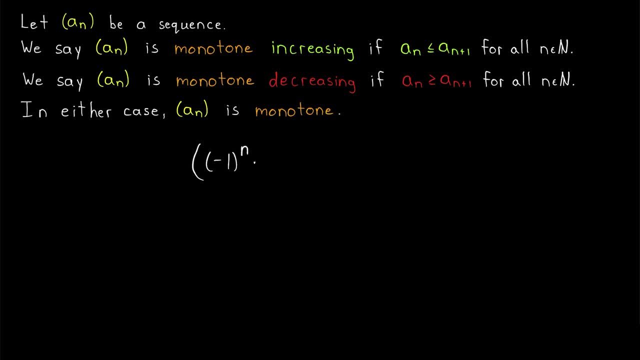 where the nth term is equal to negative one, to the power of n times n. the terms of this sequence are negative one, then positive two, then negative three, then positive four, and so on, So we get the 4 and so on. This sequence certainly isn't increasing since, for example, the second term 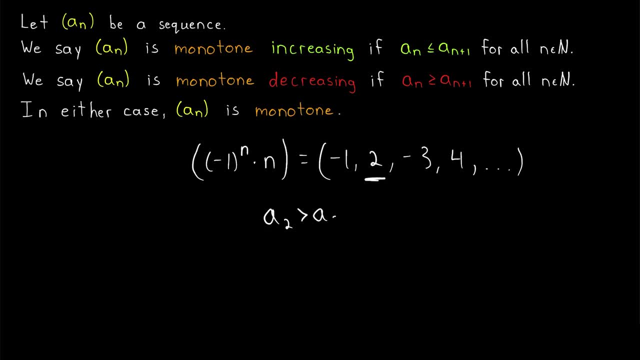 a2 is greater than the third term, a3, and to be increasing every term has to be less than or equal to the next one. Similarly, this sequence cannot be decreasing because, for example, the first term, a1, is less than the second term, a2, and for a sequence to be decreasing every term. 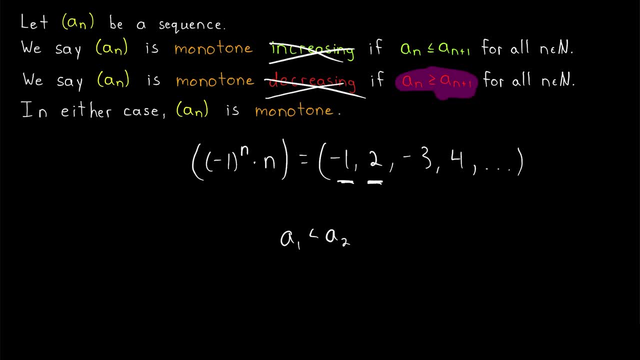 has to be greater than or equal to the next one. So this sequence is not monotone. How about the sequence where the nth term is equal to 1 over n? So the terms of the sequence are 1 over 1,, then 1 over 2, then 1 over 3, and so on. In this case, every term. 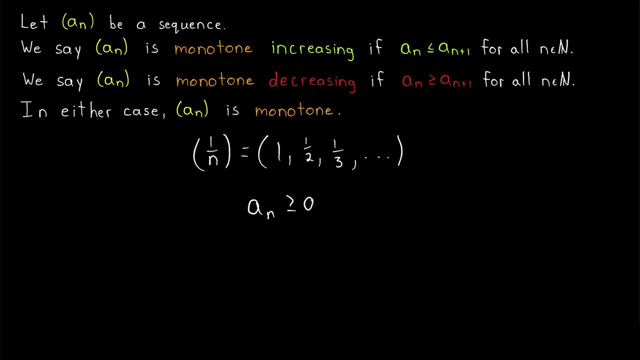 a n is indeed greater than or equal to the next term, a n plus one, And so this sequence is decreasing. we could prove that by noting that n plus one is greater than n, and then invert both sides of the inequality, giving us that one over n plus one is less than one over n. And then this: 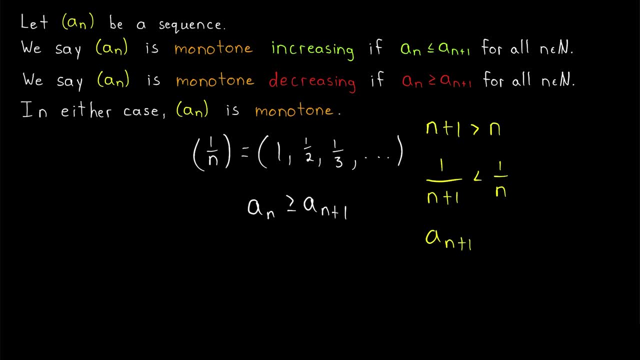 is the definition of a n plus one. this is the definition of a n, and we'd have that each term. a n is greater than a n plus one, So certainly a n is greater than or equal to a n plus one. we could also say that this sequence is strictly decreasing because, as we just saw, we could erase 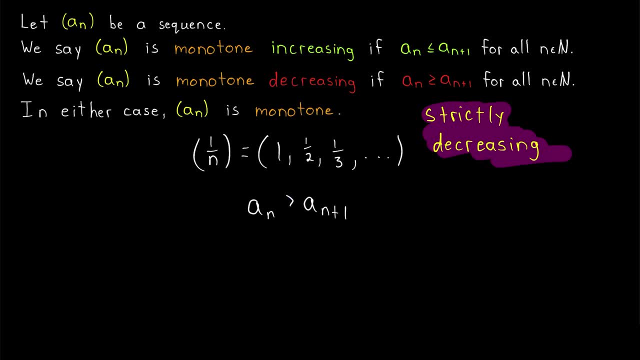 the or equal to part of this inequality, and it would still be true. Every term is greater than the next one. the terms of a decreasing sequence are allowed to not change or go down in value. For a strictly decreasing sequence, each term has to be going. 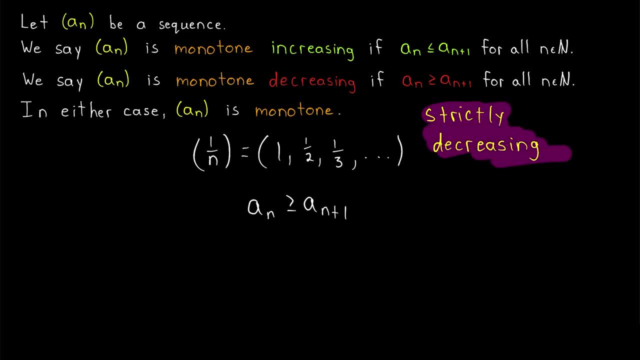 we could also say that this sequence is strictly decreasing because, as we just saw, we could erase the or equal to part of this inequality, and it would still be true: Every term is greater than the next one. the terms of a decreasing sequence are allowed to. 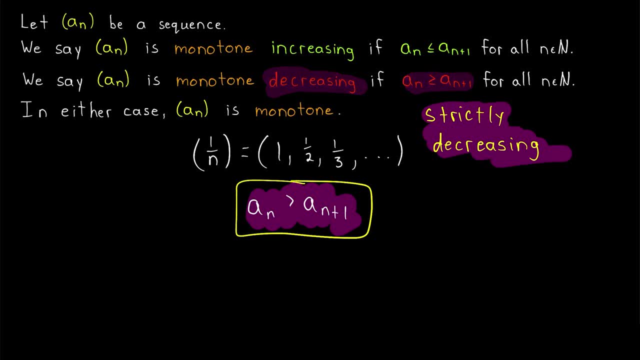 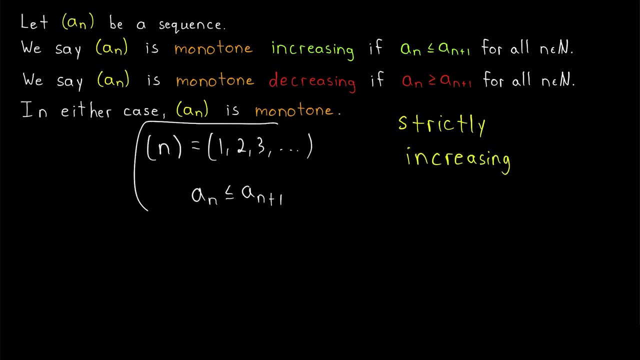 not change or go down in value For a strictly decreasing sequence. each term has to be going down. they have to be strictly decreasing. Similarly for sequences that we would call strictly increasing. this sequence we looked at earlier is strictly increasing because not only 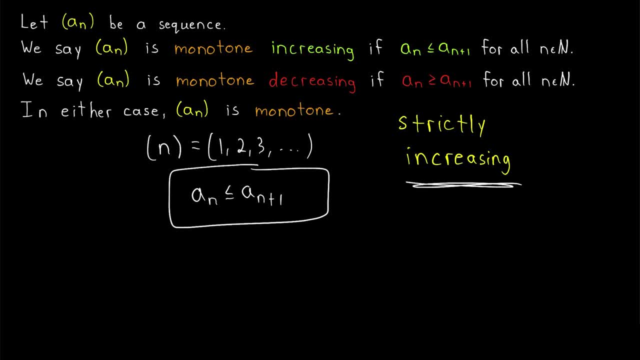 is every term greater than or equal to a n plus one, but every term is greater than or equal to the next one, but every term is less than the next one. Sometimes these sorts of sequences are also called strictly monotone, where every term is either getting bigger, which is strictly increasing, 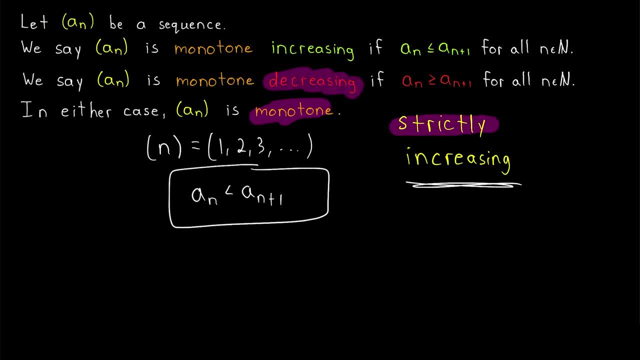 or every term is getting smaller, which is strictly decreasing. Usually these more general definitions work for us, but you will occasionally encounter the strictly variance as well. Here's one more weird example: 1 squared over 2 to the n. the terms of this sequence are 1 squared over 2 to the one, so that's. 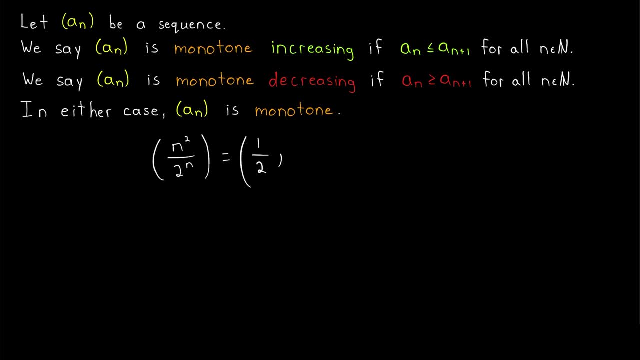 one half, then two, squared over two, to the power of two, which is four, over four, which is one, then three, squared, which is nine, over two, to the power of three, which is eight, then four squared, which is 16, over two to the power of four, which is 16.. So that's just one then five. 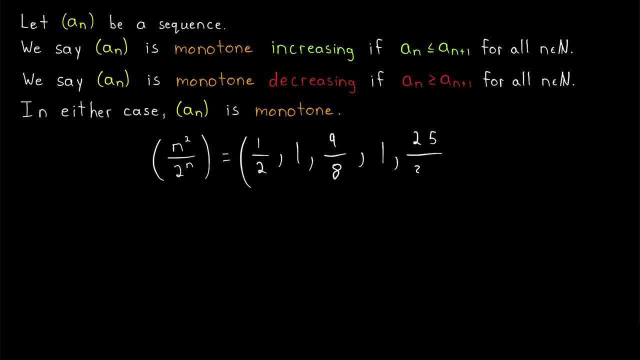 squared, which is 25, over two, to the power of five, which is 32,, then six squared, which is 36,, over two to the power of six, which is 64, and so on. This sequence is certainly not increasing. 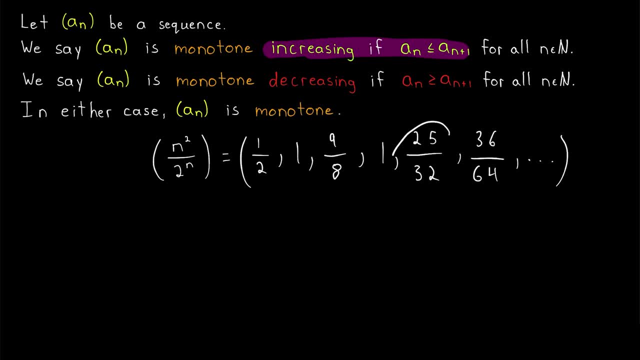 since, for example, this term is greater than the next term, but it's also not decreasing, since, for example, this term is less than the next term. So here the sequence gets bigger for just a second, and then here the sequence gets smaller. So this sequence is not. 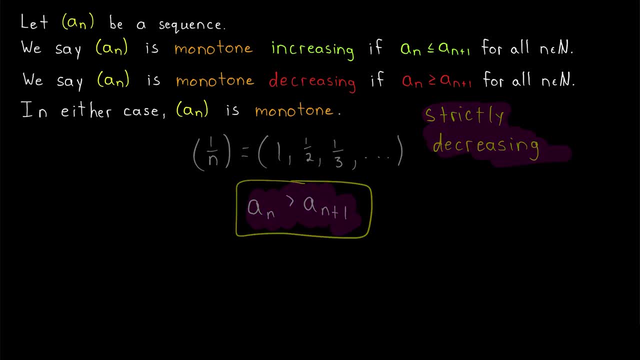 down. they have to be strictly decreasing. Similarly for sequences that we would call strictly increasing. this sequence we looked at earlier is strictly increasing, because not only is every term a n plus one, but every term is a n plus one, And so this is the definition of a n. 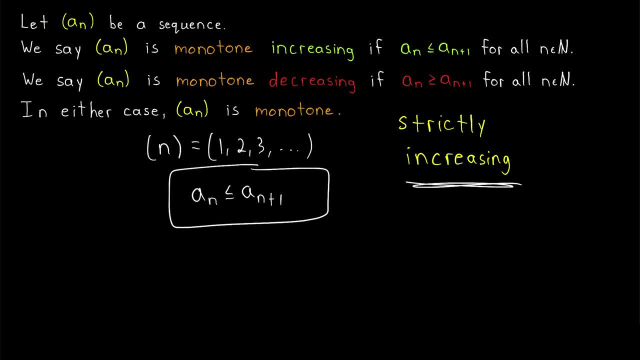 less than or equal to the next one, but every term is less than the next one. Sometimes these sorts of sequences are also called strictly monotone, where every term is either getting bigger, which is strictly increasing, or every term is getting smaller, which is strictly decreasing. 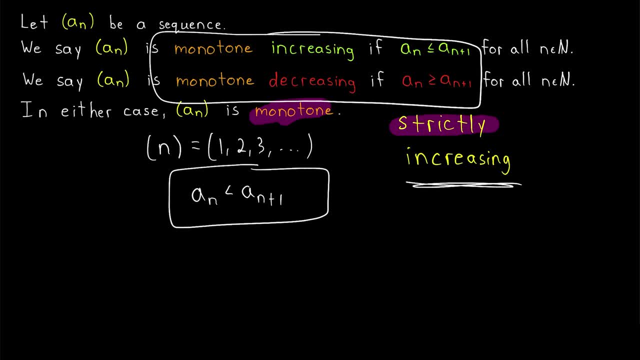 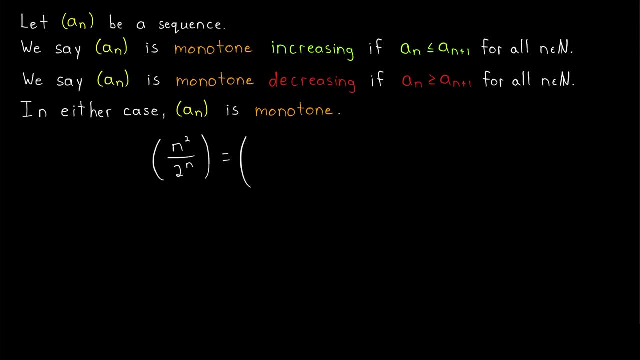 squared over two to the n. the terms of this sequence are one squared over two to the one, So that's one half, then two squared over two, to the power of two, which is four over four, which is one, then three. squared which is nine over two to the power of three, which is eight, then four. 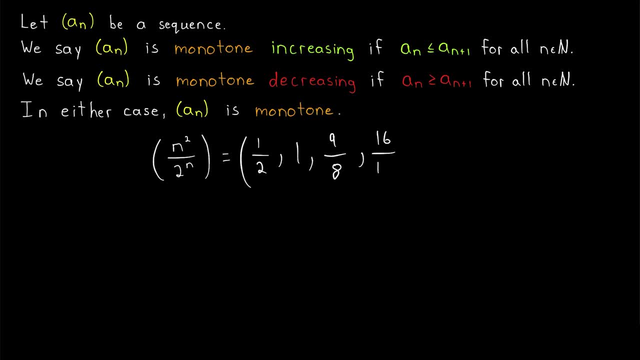 squared, which is 16, over two, to the power four, which is 16.. So that's just one. then five squared, which is 25, over 2, to the power of 5,, which is 32,. then 6 squared, which is 36, over 2, to the. 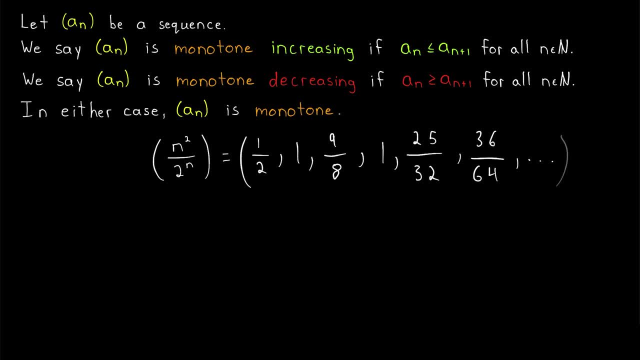 power of 6, which is 64, and so on. This sequence is certainly not increasing, since, for example, this term is greater than the next term, but it's also not decreasing, since, for example, this term is less than the next term. So here the sequence gets bigger for just a second, and then here the 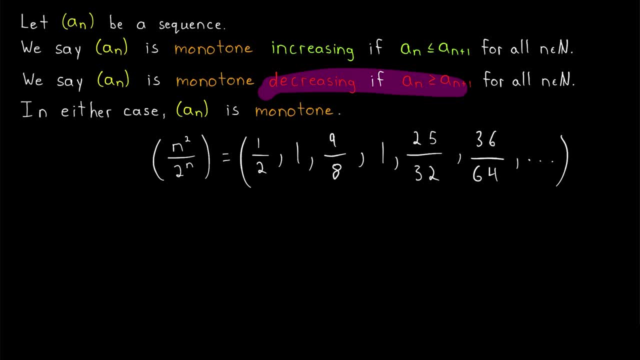 sequence gets smaller. So this sequence is not monotone, but it does have another interesting property. This is a sequence that we would say is eventually decreasing, Although it behaves a little weirdly at the beginning. from this point onwards, the sequence will just get smaller and 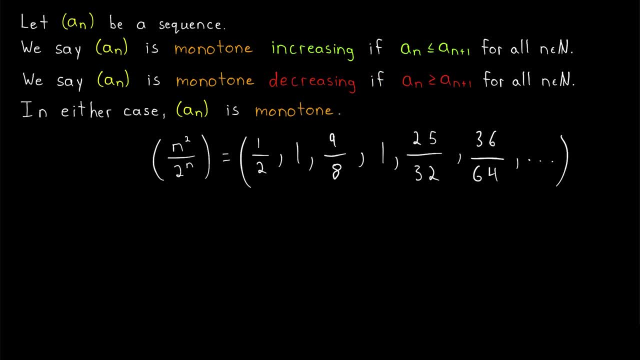 monotone. but it does have another interesting property. This is a sequence that we would say is eventually decreasing, Although it behaves a little weirdly at the beginning. from this point onwards the sequence will just get smaller and smaller. So we say it is eventually decreasing. 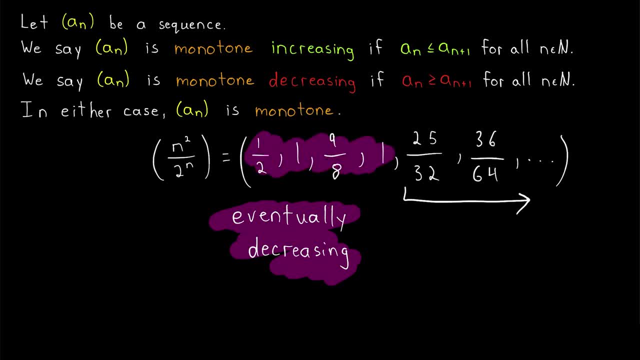 because after a finite number of turns the sequence behaves like a decreasing sequence. And of course you could state a similar definition for eventually increasing sequences. And in general we say that a sequence eventually has property x if it has property x after a finite number of turns. Again, it is these more. 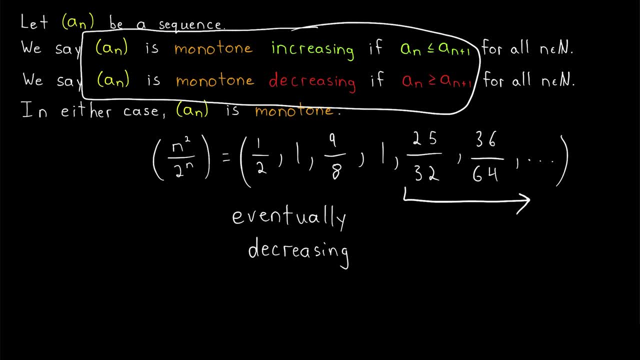 general definitions of a monotone sequence that we'll be most interested in, but it's good to be aware of the variance, Strictly and eventually. The first big theorem that will prove about monotone sequences is really cool. It's called the monotone convergence theorem and it concerns sequences that are both monotone and bounded. 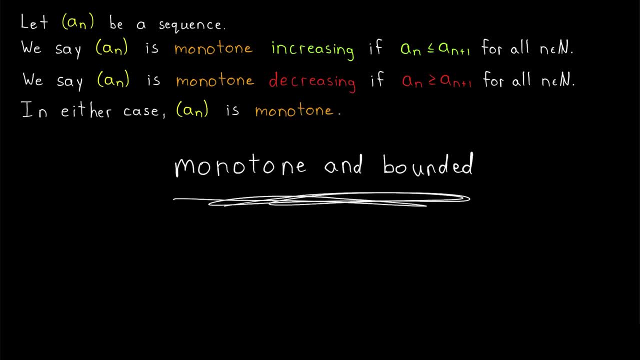 What do you think we can say about a monotone and bounded sequence? Remember, monotone means it's increasing or decreasing Or, as we saw, it could be both if it's a constant sequence. So among the sequences have been monot alcoholic and monotlerde. 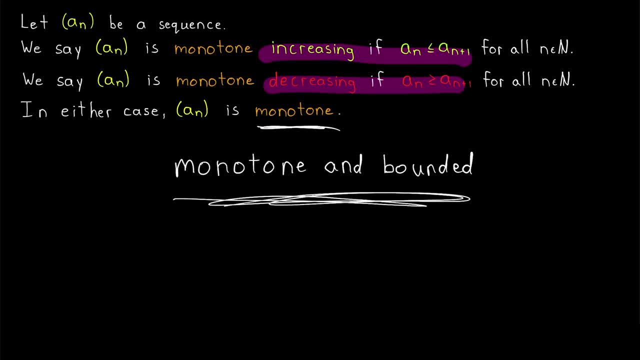 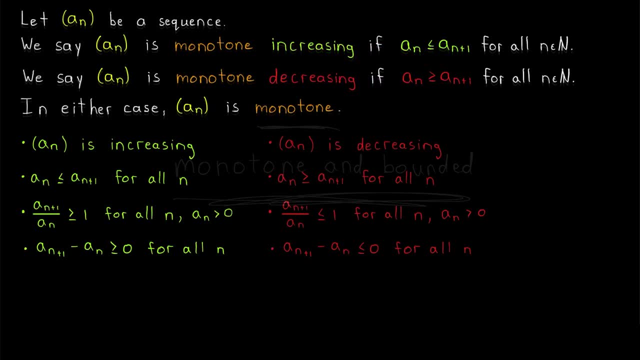 I'll leave a link in the description to the lesson where we prove the monotone convergence theorem, which will tell us everything we need to know about monotone and bounded sequences. One last thing: here's a list of equivalent ways to characterize that a sequence is increasing. 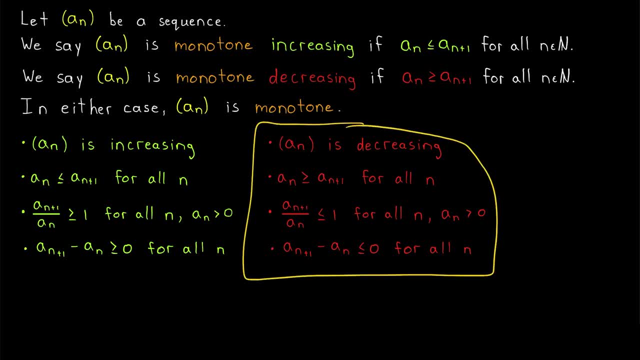 and here are some equivalent ways to characterize that a sequence is decreasing. The first two bullet points are basically just our definitions. Increasing means every term is less than a constant equation. Decreasing means every term is less than or equal to the next one. 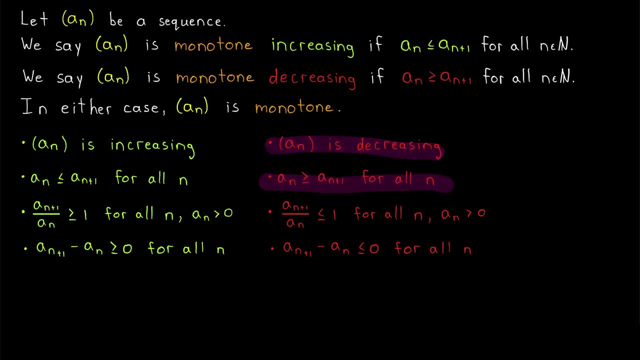 Decreasing means every term is greater than or equal to the next one. The second bullet point in each list gives us the fourth bullet point by just subtracting across the inequality. The third bullet points are a little bit trickier. For an increasing sequence, the ratio of a term to the previous term is greater than. 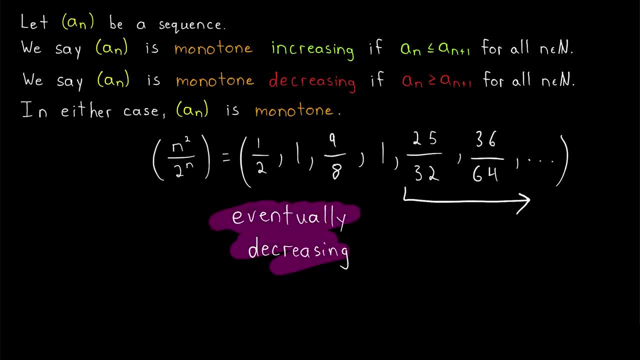 smaller. So we say it is eventually decreasing. Decreasing because after a finite number of terms the sequence behaves like a decreasing sequence. And of course you could state a similar definition for eventually increasing sequences. And in general we say that a sequence eventually has property x if it has property x after a finite. 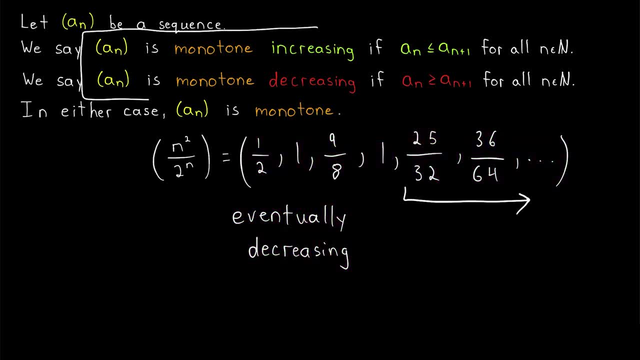 number of terms. Again, it is these more general definitions of a monotone sequence that will be most important. The first big theorem that will prove about monotone sequences is really cool. It's called the monotone convergence theorem and it concerns sequences that are both monotone and bounded. 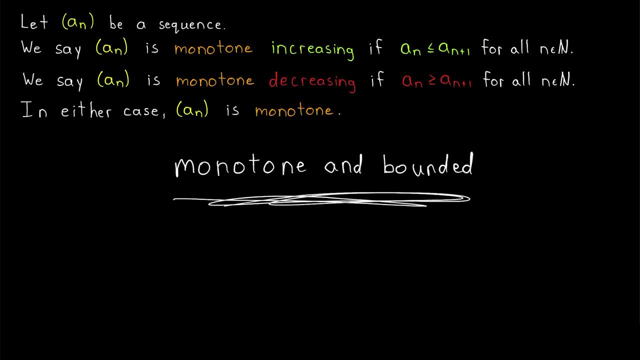 What do you think we can say about a monotone and bounded sequence? Remember, monotone means it's increasing or decreasing Or, as we saw, it could be both if it's a constant sequence. I'll leave a link in the description to the lesson where we prove the monotone convergence theorem. 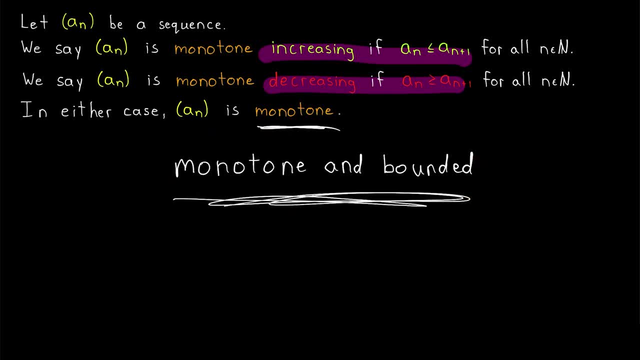 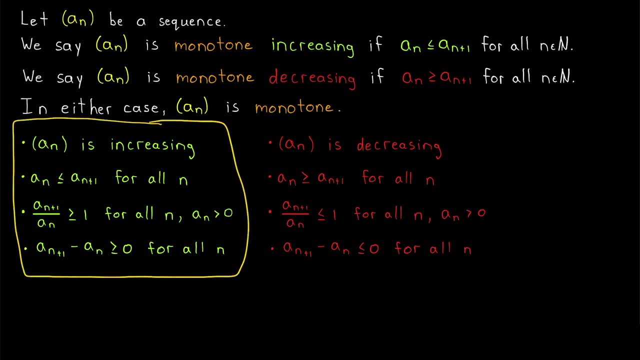 which will tell us everything we need to know about monotone and bounded sequences. One last thing: Here is a list of equivalent ways to characterize that a sequence is increasing, and here are some equivalent ways to characterize that a sequence is decreasing. The first two bullet points are basically: 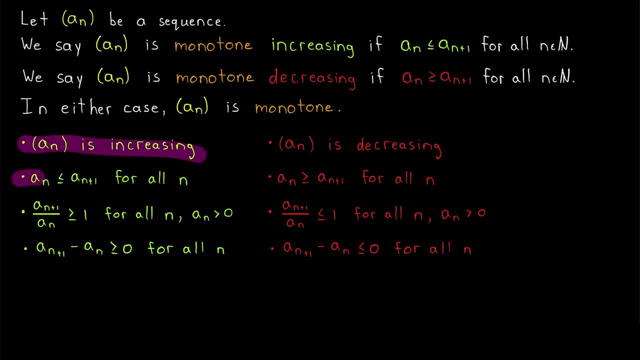 just our definitions. Increasing means every term is less than or equal to the next one. Decreasing means every term is greater than or equal to the next one. The second bullet point in each list gives us the fourth bullet point by just subtracting across the inequality. 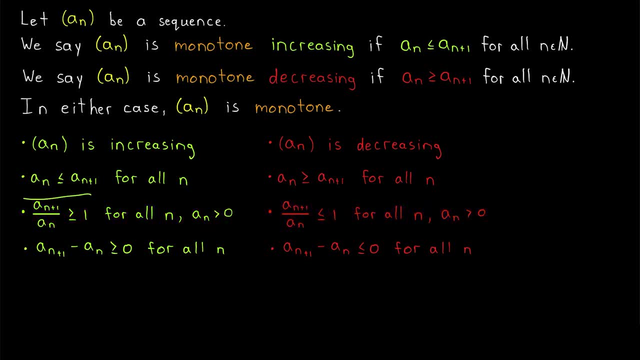 The third bullet points are a little bit trickier. For an increasing sequence, the ratio of a term to the previous term is greater than or equal to one, provided all the terms are equal And all the terms are greater than zero. If some of the terms are negative, then for an increasing sequence, for example, 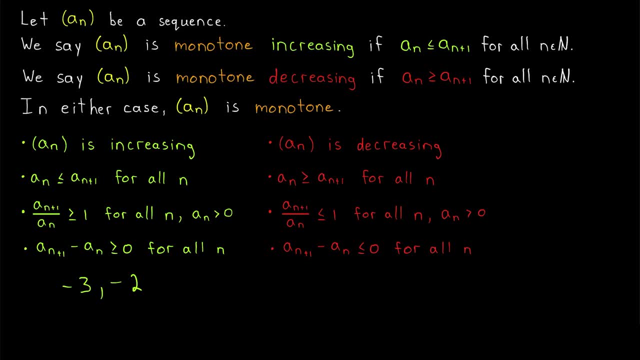 we could go from negative three to negative two, in which case the ratio of one term to the previous term is equal to two-thirds, which is less than one, And we have a similar property for decreasing sequences: The ratio of a term to the previous term is less than or equal to one for a decreasing sequence. 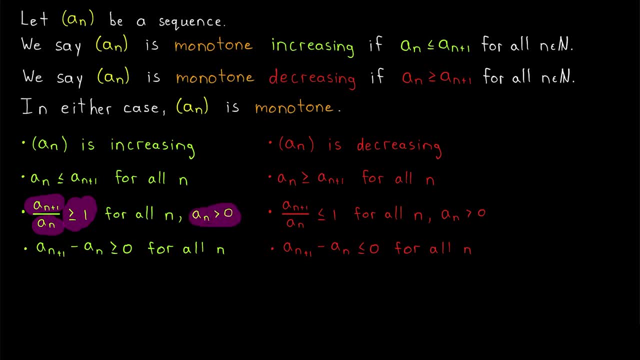 or equal to one, provided all the terms are greater than zero. If some of the terms are negative, then for an increasing sequence. for example, we could go from negative three to negative two, in which case the ratio of one term to the previous. 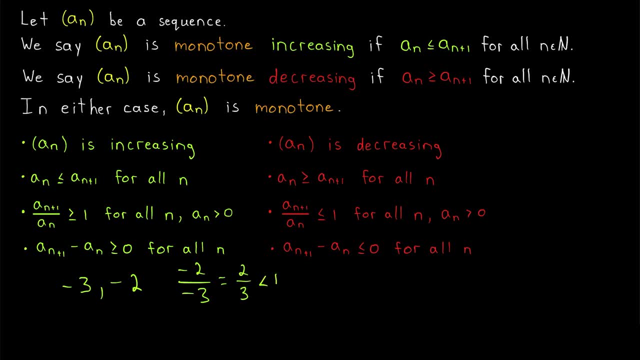 term is equal to two thirds, which is less than one, And we have a similar property for decreasing sequences. The ratio of a term to the previous term is less than or equal to one For a decreasing sequence, provided that all terms of the sequence are positive. 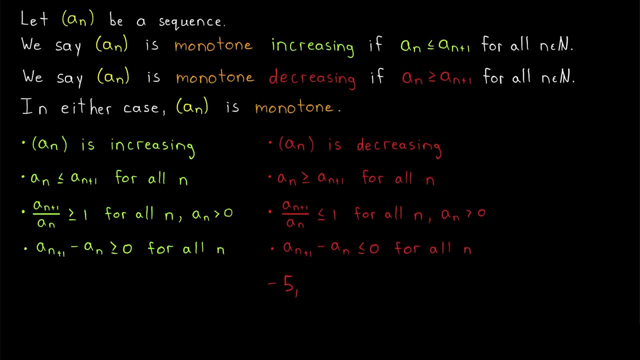 For a decreasing sequence. it could go from negative five to negative ten, And then the ratio of one term to the preceding term would be positive two which is greater than one, And of course, in either case, we can't be dividing by zero. 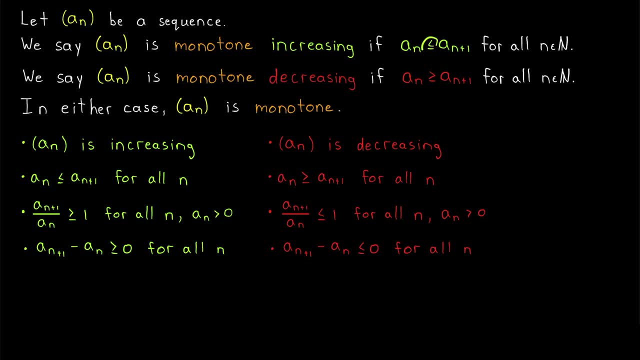 The final thing I'd like to point out before we go. since less than or equal to is a transitive relation, we don't just have that a n is less than or equal to a n plus one for an increasing sequence. We could also say that a n is less than or equal to a m whenever m is greater than or. 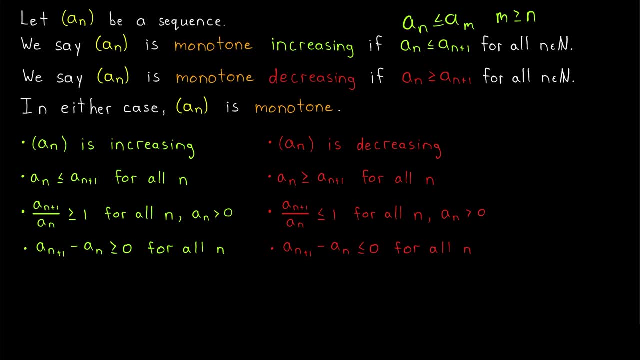 equal to n. So, for example, this could be a n and this could be a n plus 100.. Certainly, in an increasing sequence, a term has to be less than or equal to a term that comes after it. No, It's not just the term that immediately comes after it. 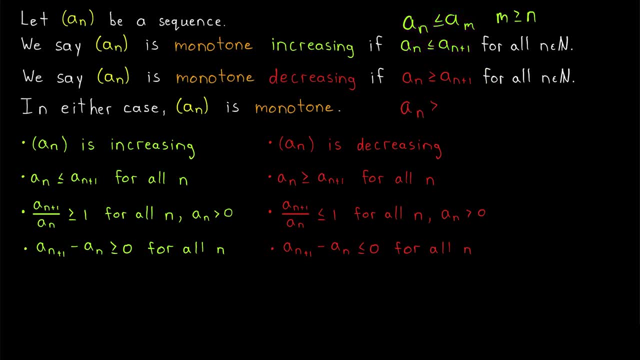 Similarly for decreasing sequences, we could say that a n is greater than or equal to a m. provided that m is greater than or equal to n, Any term in a decreasing sequence is greater than or equal to any term that comes after it, not just the term that comes immediately after it. 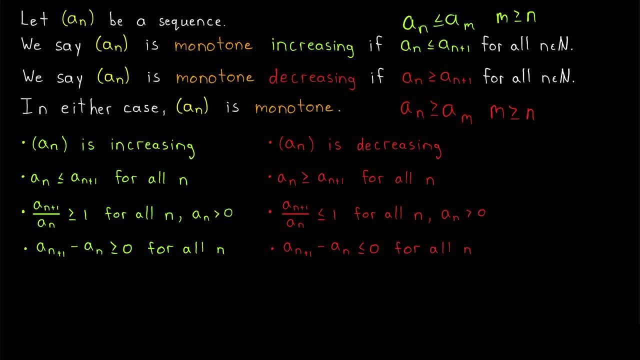 So that's a quick look at monotone sequences. Remember a sequence can be increasing Or decreasing. In either case, we call it monotone. I hope the examples and some of the related definitions were helpful. Let me know if you have any questions.